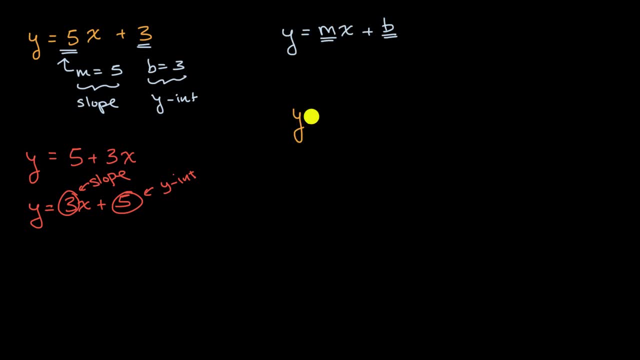 Let's say that we have the equation: y is equal to 12 minus x. Pause this video and see if you can determine the slope and the y-intercept. All right, so something similar is going on here that we had over here: The standard form, slope-intercept form. 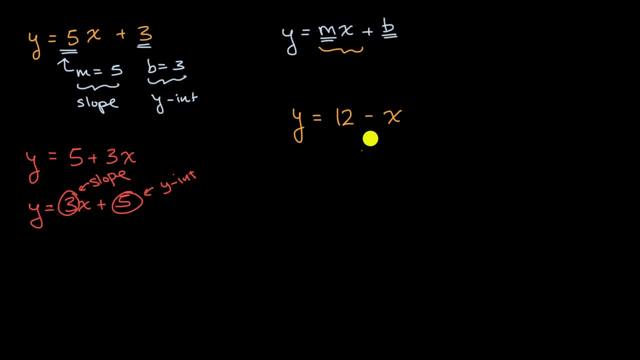 we're used to seeing the x term before the constant term, so we might want to do that over here. So we could rewrite this as: y is equal to negative x plus 12,, negative x plus 12.. And so from this you might immediately recognize: 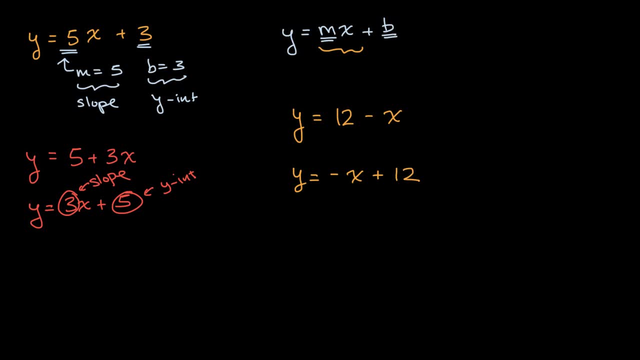 okay, my constant term when it's in this form: that's my b, that is my y-intercept. so that's my y-intercept right over there. but what's my slope? Well, the slope is the coefficient on the x term. 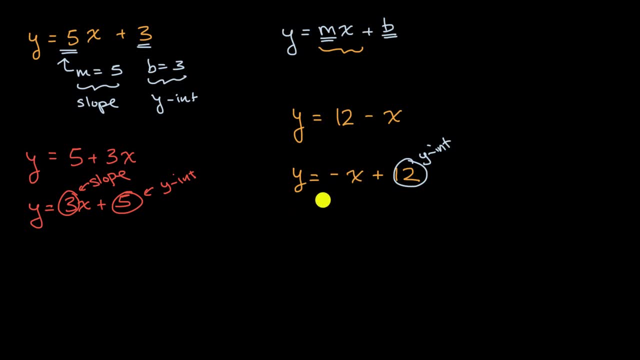 but all you see is a negative here. What's the coefficient? Well, you could view negative x as the same thing as negative one x. so your slope here is going to be negative one. Let's do another example. Let's say that we had the equation: y is equal to five x. 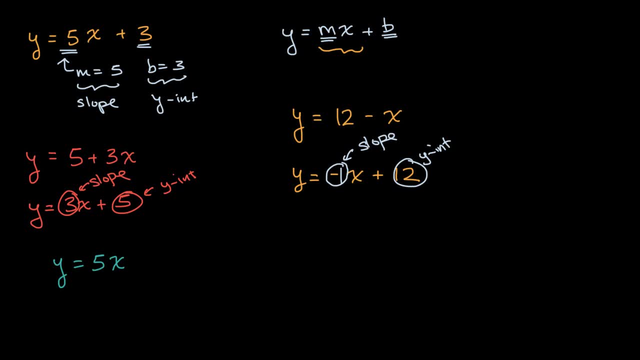 What's the slope and y-intercept there? At first you might say, hey, this looks nothing like what we have up here. This is only. I only have one term on the right-hand side of the equality sign. Here I have two. 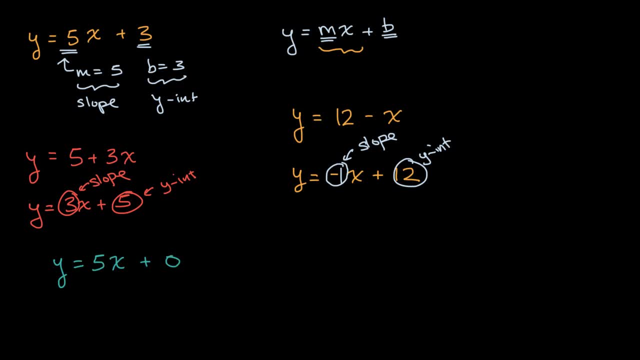 But you could just view this as five x plus zero, and then it might jump out at you that our y-intercept is zero and our slope is the coefficient on the x term. It is equal to five. Let's do one more example. 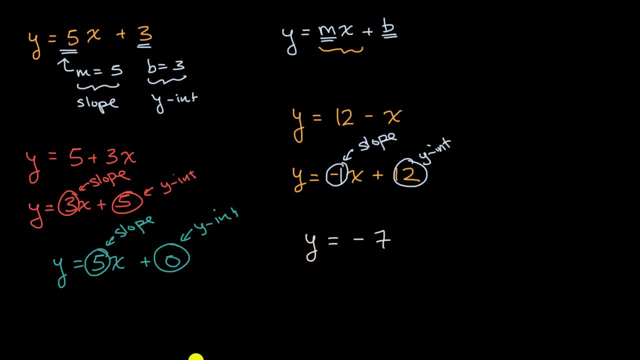 Let's say we had: y is equal to negative seven. What's the slope and y-intercept? It's the y-intercept there. Well, once again you might say, hey, this doesn't look like what we had up here. 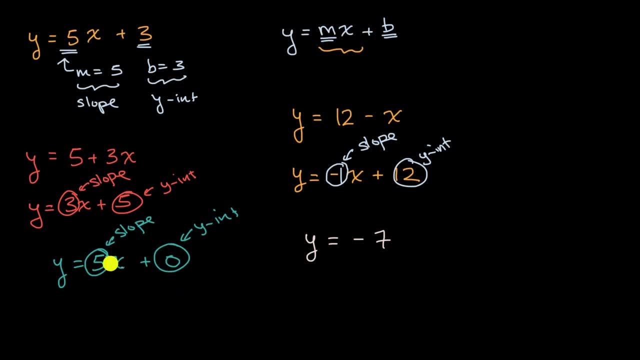 How do we figure out the slope or the y-intercept? Well, we could do a similar idea. We could say: hey, this is the same thing, as y is equal to zero times x minus seven, And so now it looks just like what we have over here. 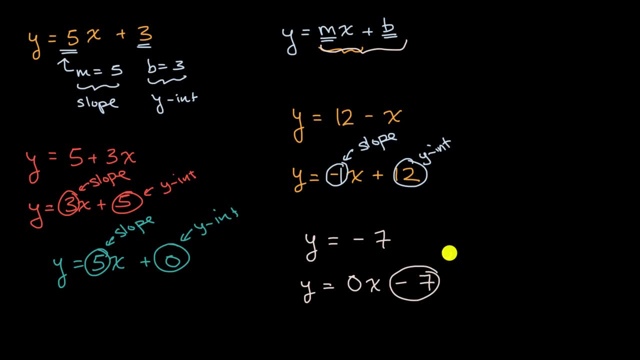 and you might recognize that our y-intercept is negative seven. Y-intercept is equal to negative seven And our slope is a coefficient. on the x term It is equal to zero And that makes sense. For a given change in x you would expect zero change in y.